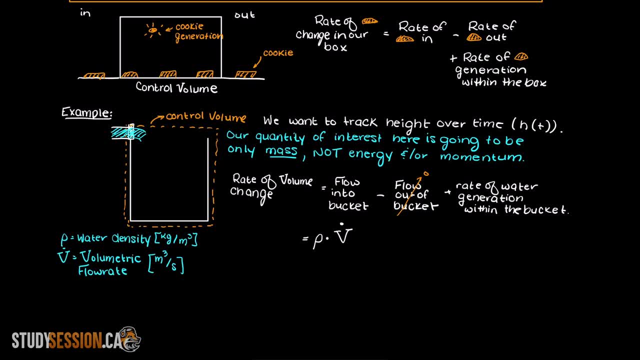 give the units of kilograms per second. We also know that we will have no generation or consumption term here, as there is no water being generated or consumed in our control volume. Lastly, we need to determine the rate of change of our water term, So the rate of volume change within. 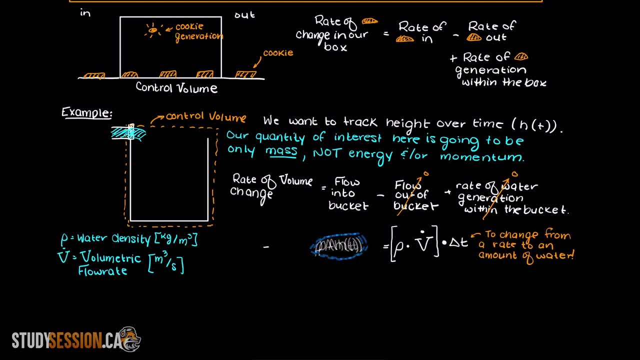 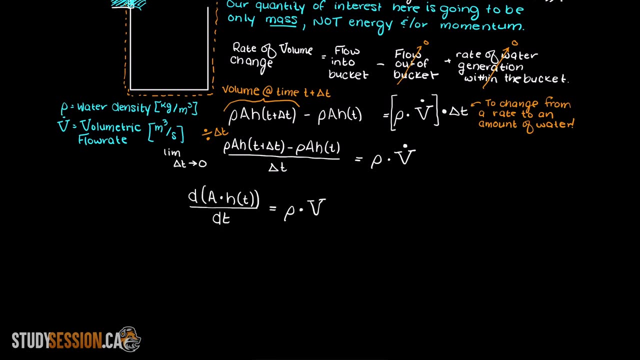 our bucket will be the volume at some time, t subtracted from the volume at some time slightly further into the future. Now, if we divide by our small increment in time, we can take the time as it approaches zero and we get the first order derivative rate of change of our volume within. 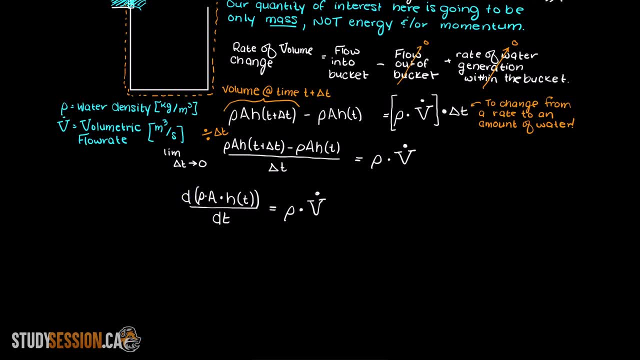 the bucket, which is almost what we want. Let's also recognize something. The volume of something can be found through the density times, the area times, the height of the liquid. Additionally, since the area and density are considered constant, they are not going to change with time. We can. 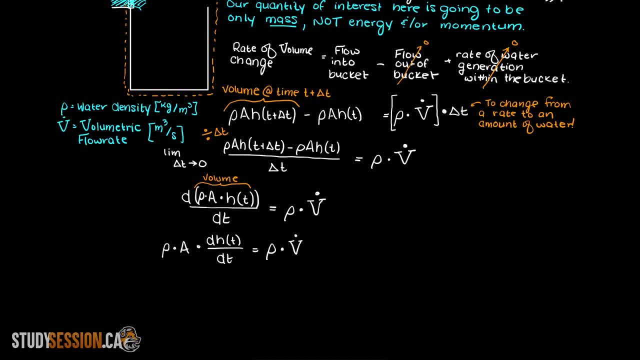 bring both these terms outside the time derivative. Lastly, we can divide out these terms and we are left with the rate of change in our bucket's height all through our balance equation, which is pretty awesome. So once we get the final answer like this, it makes sense that we should validate. 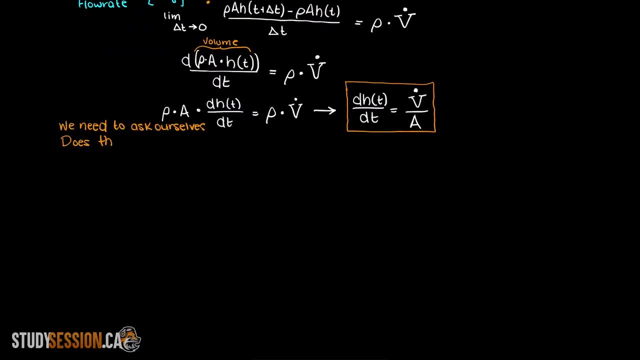 our answer right. We could do this simply by assuming all but one variable in our equation are constants and then alter the other variable and seeing if it makes sense. Through this you can quickly understand if your newly found derivative actually makes sense. Here there are only two time. 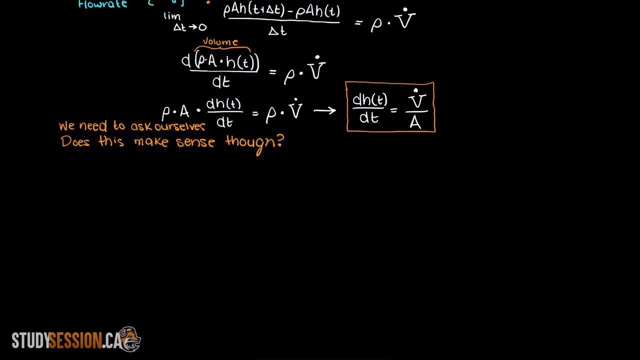 variables. However, this would work if we were to divide by the number of times. a variable is constantly variable, So here lets assume that the area is constant. Then lets say that we increase our flowrate into our bucket. Will this increase or decrease the rate of change in the? 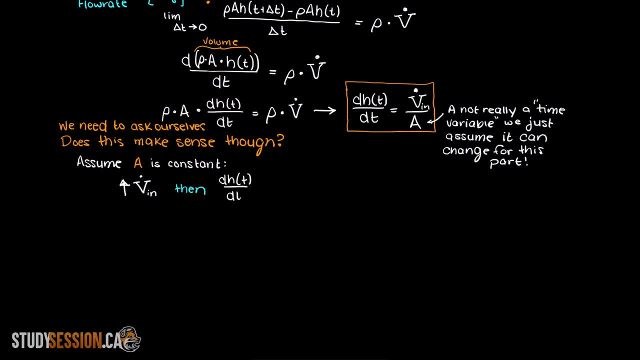 height over time. Well, it will increase, which it should, and this makes sense. Additionally, we could ask what would happen if we decreased it? Well then, the rate of height change with time would decrease, which also makes sense. What if we changed the? 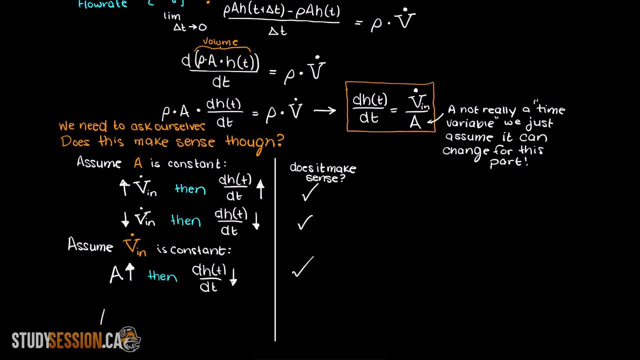 area over time to 0?. Well then, we could change it by the number of times the area was constantly bucket and kept the flow rate into our control volume the same, While with a larger area it would only make sense for the rate of change of the height.